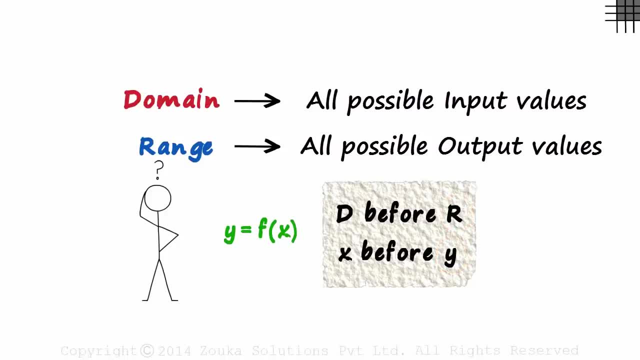 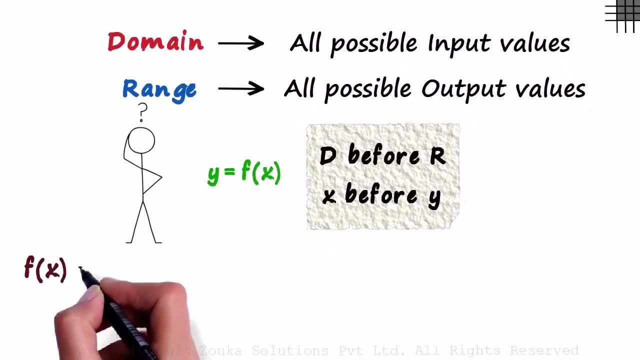 Domain is x and the range is y. Ok, nice Shall we try out a few examples now. The first function is: f of x is equal to x. This function will simply give out the value it takes as the input, Instead of saying it does nothing. 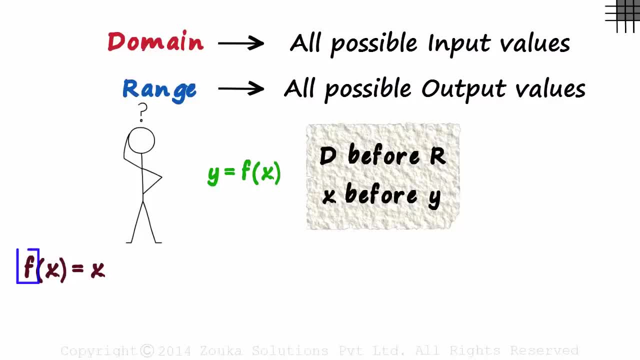 A better way of saying it is to say: f of x is equal to x. This function will simply give out the value it takes as the input, And the way of doing it would be: the function multiplies the input by one and gives an output. 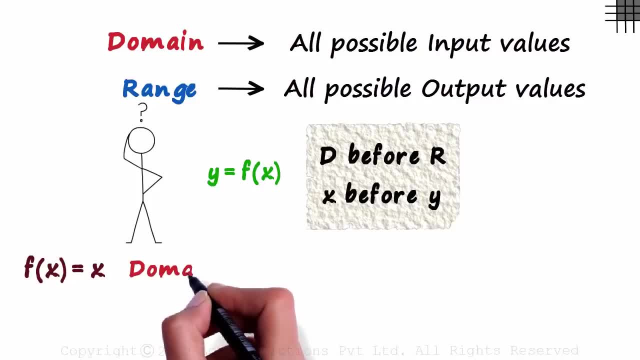 Anyway, coming to the point, what will be the domain and the range of this function? Domain will be all the values x can take In this function. x can take any value, Yes, just about any value. So the domain is all x. 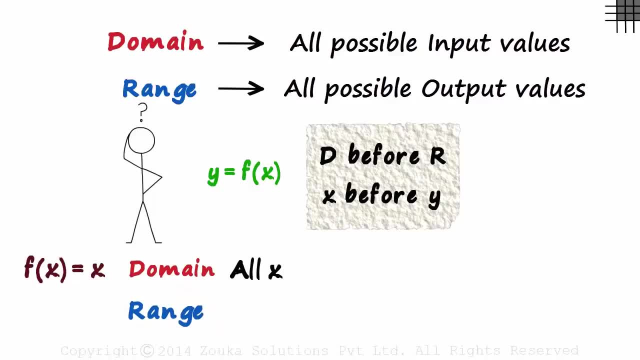 And the range, which is y, or the output, can also take all values that x takes. So the range will be all y values. Here's the second function: f of x is equal to x squared. What will be the domain and the range of this function? 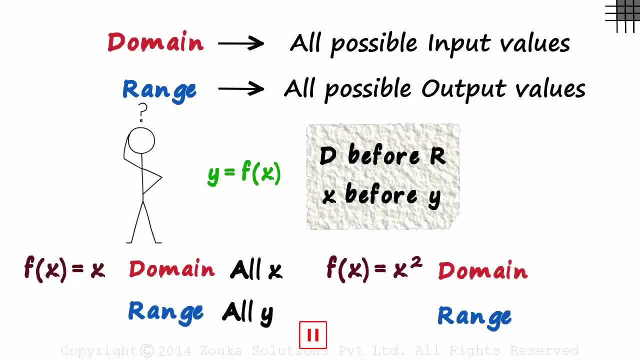 Try it out. The input x can take any value, So the domain will be all x. The range is interesting. Will it be all y? It will be all y greater than or equal to zero. Why? Because the square of any number cannot be negative. 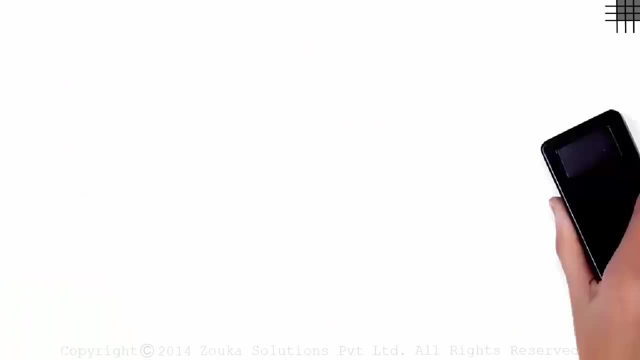 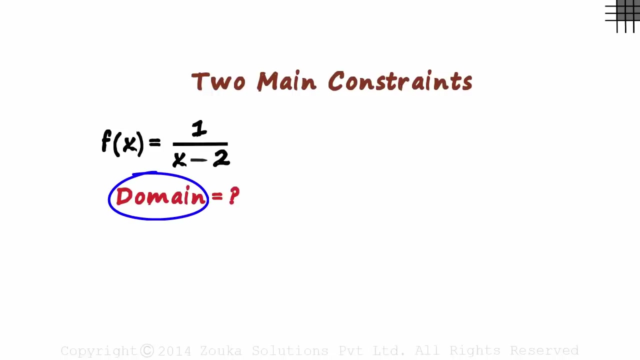 It will always be non-negative. To give you some good news, there are two main constraints that are very common in the exams. Look at this function: f of x is one over x minus two. What is the domain of this function? Domain is the set of all possible input values. 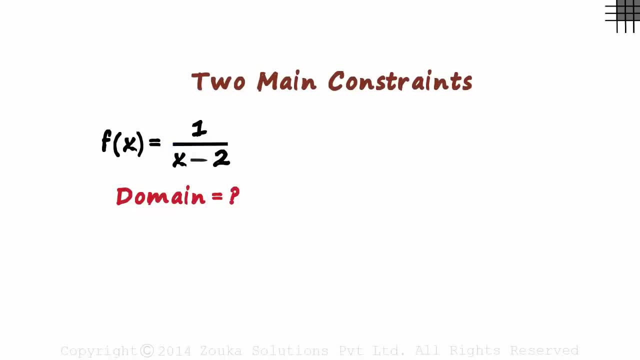 Can x take any value here? Yes, all but one value. The domain will be all x except x equal to two. That's the first constraint. The denominator has to be a non-zero, Because if it is a zero then the function will be undefined. 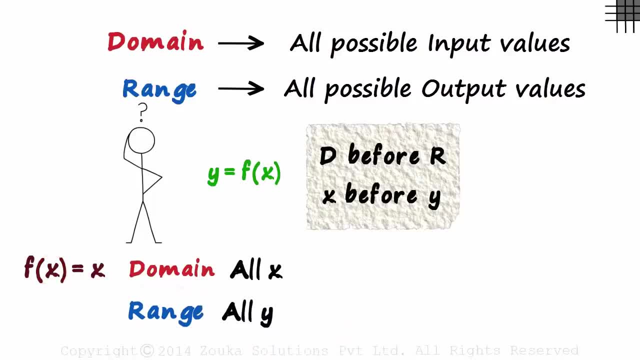 So the range will be all y values. Here's the second function. f of x is equal to x squared. What will be the domain and the range of this function? Try it out. The input x can take any value, So the domain will be all x. 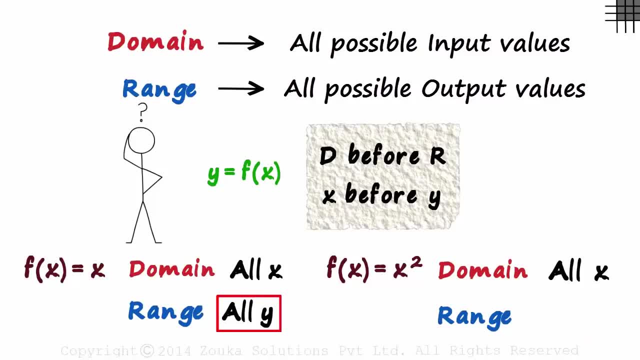 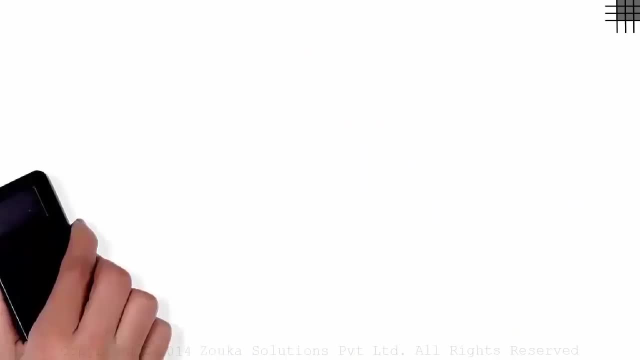 The range is interesting. Will it be all y? It will be all y greater than or equal to zero. Why? Because the square of any number cannot be negative. It will always be non-negative. To give you some good news, there are two main constraints that are very common in the exams. 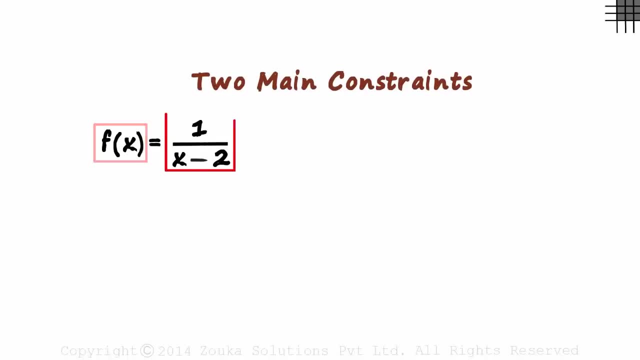 Look at this function: f of x is 1 over x minus 2.. What is the domain? What is the domain of this function? Domain is the set of all possible input values. Can x take any value here? Yes, all but one value. 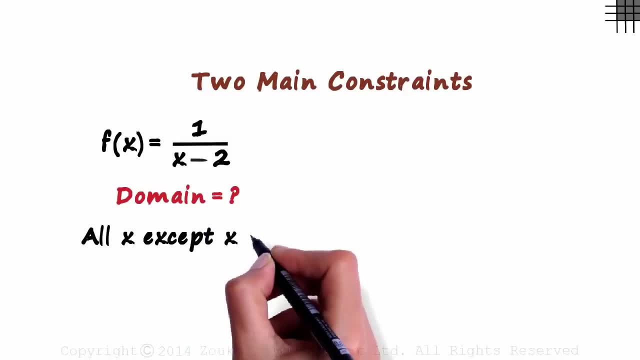 The domain will be all x except x equal to 2.. That's the first constraint. The denominator has to be a non-zero, Because if it is a zero then the function will be undeniable, It will be undefined. Easy, Here's another one. 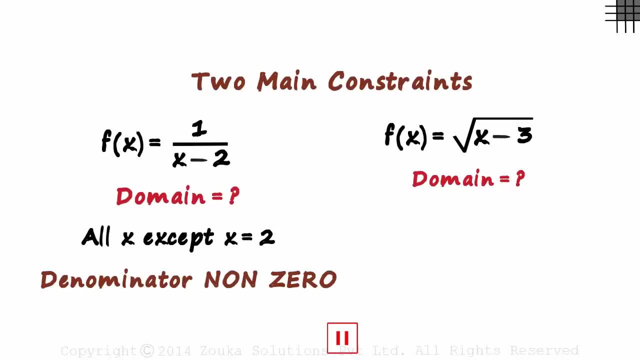 What is the domain of this function? Can we have a negative number within the square root? Well, I don't think we can. So x minus 3 will be greater than or equal to zero. This means x has to be greater or equal to 3.. 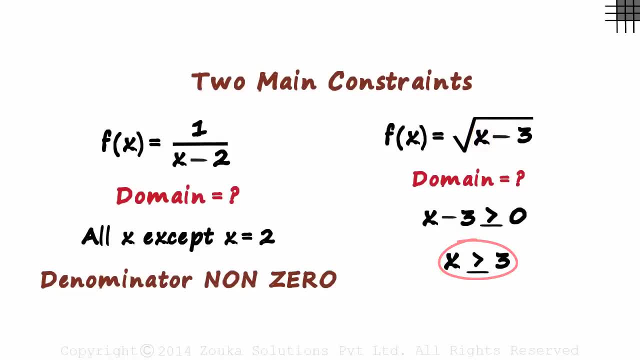 x can take any value which is greater than or equal to zero. This means x has to be greater or equal to 3.. That brings us to the second constraint. Even roots can have only non-negative numbers under them. Remember this well. The denominator has to be a non-zero.